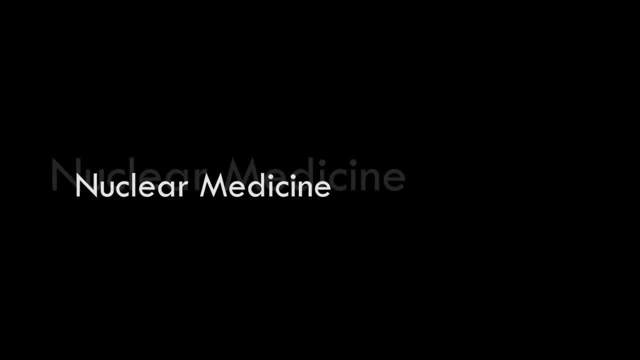 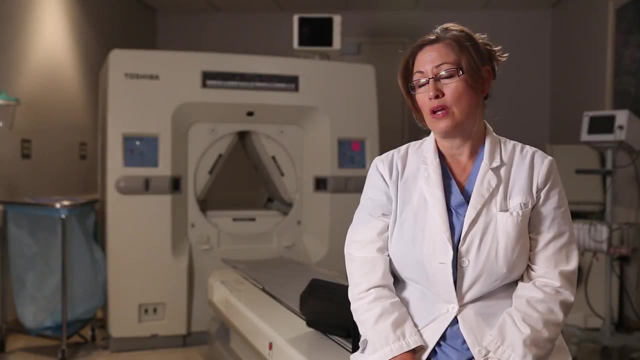 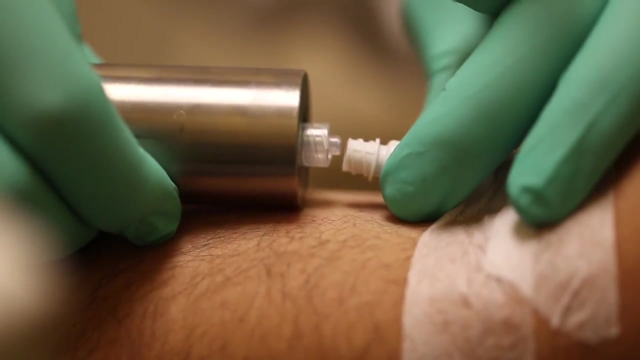 Nuclear medicine is the study of the function of organs. What we do is we inject a radioactive medicine into the blood and then we're able to image the organs and how they work and how they function. I love the fact that I work with people, The patients we actually 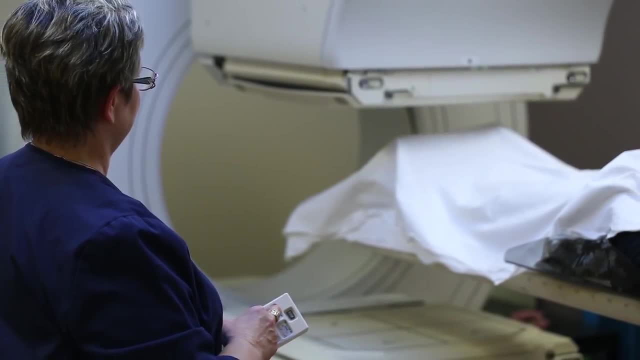 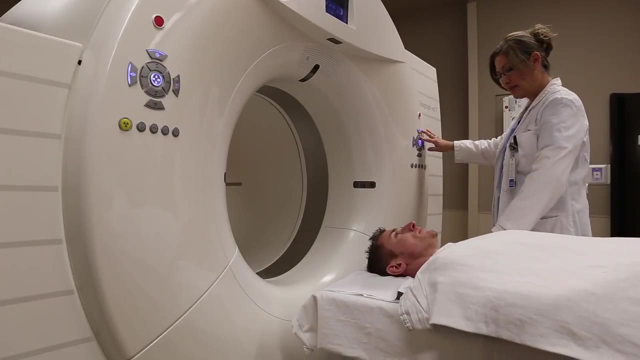 get to spend time with, whereas when you're working with x-ray, you take them in for a very quick x-ray and hold your breath. okay, breathe, you're gone. This way, our procedures take time. you get to talk to the patients. you get to teach them what you're doing, tell. 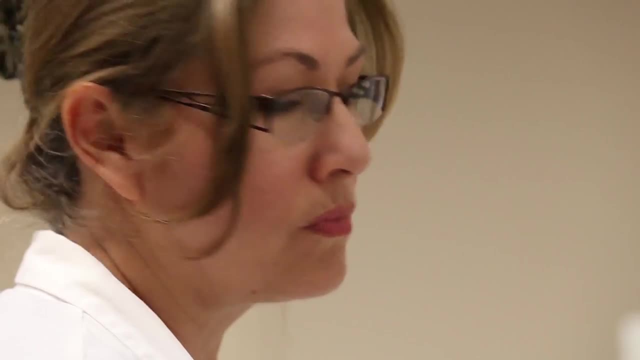 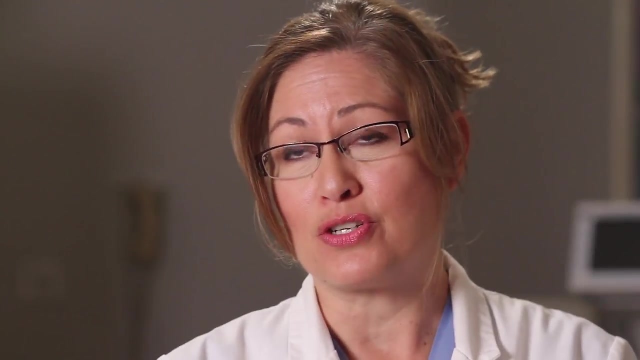 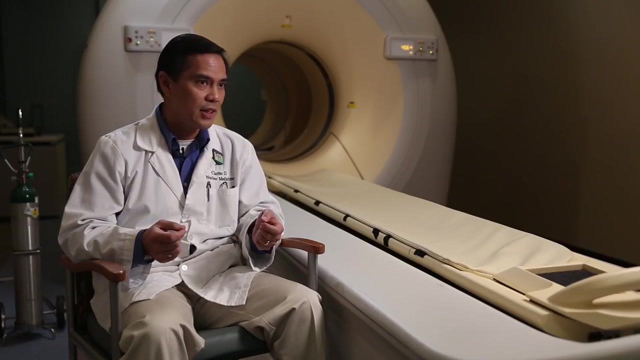 them about their procedure. I chose nuclear medicine because I really enjoy physics imaging diagnostics, which is taking the pictures, as well as working with the patients, and this really incorporates all of those things together. On the day of my studies, I usually do a. 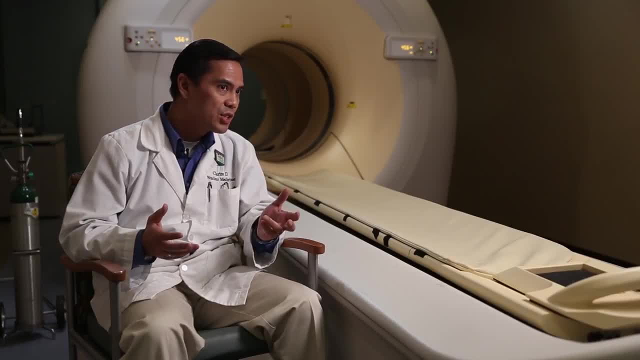 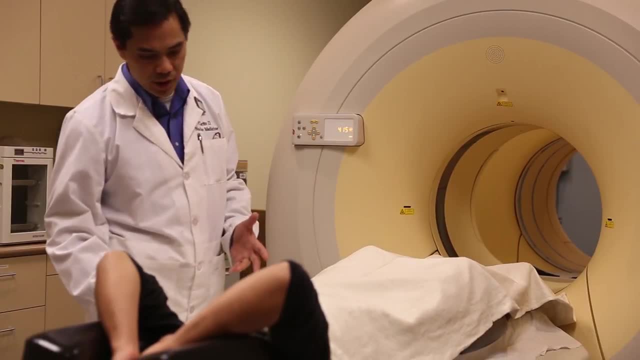 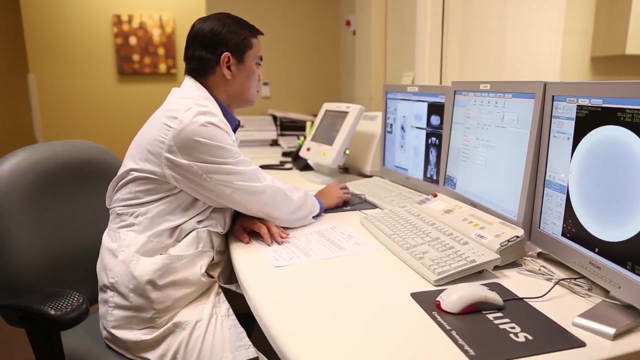 quality control, which is basically going to our machines, making sure all the machines are working properly. Then I go with my usual job: interview the patients, get their history and perform the exams. At the end of the day, I collect all the information I do enter. 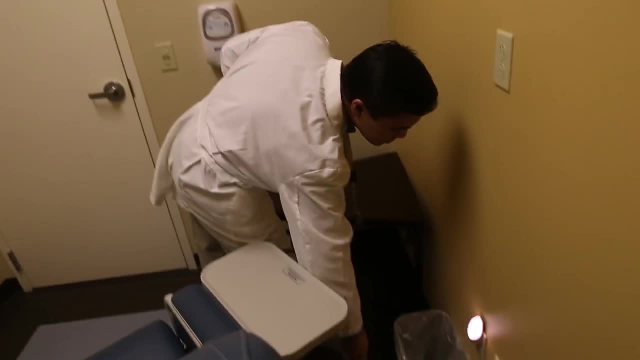 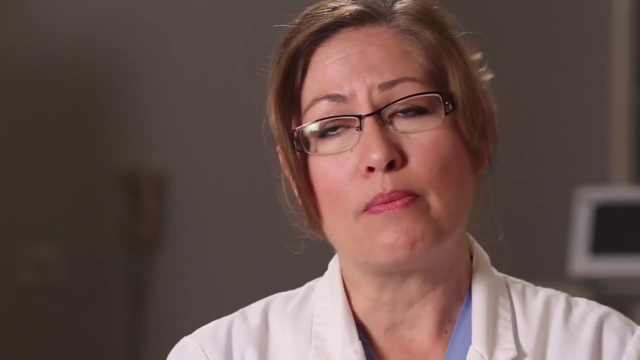 it in a computer. do my wipe down. make sure everything's still proper- no contamination. I think the most important thing is you really need to be flexible and quick on your feet. There are many ways to do different scans, but you need to be able to work and assess. 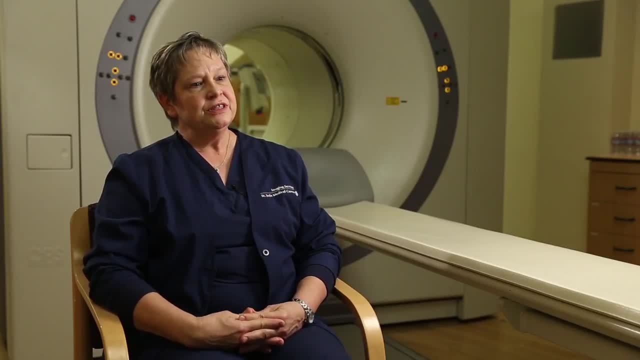 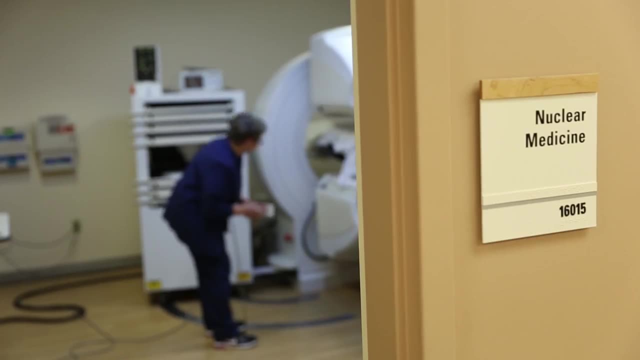 the situation. Communication is very important. You need to be able to talk to all different kinds of people: doctors, patients. You need to have some computer background, of course, a good science background, anatomy, physiology background. Sometimes, believe it or not, 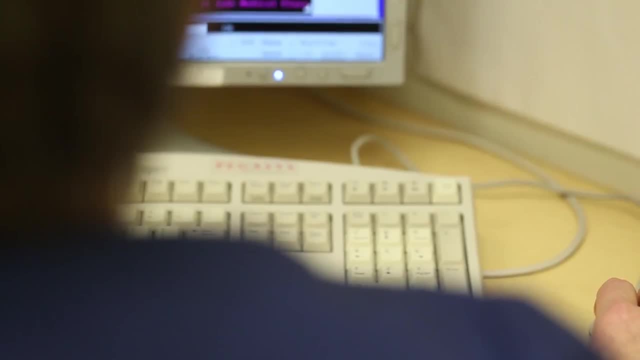 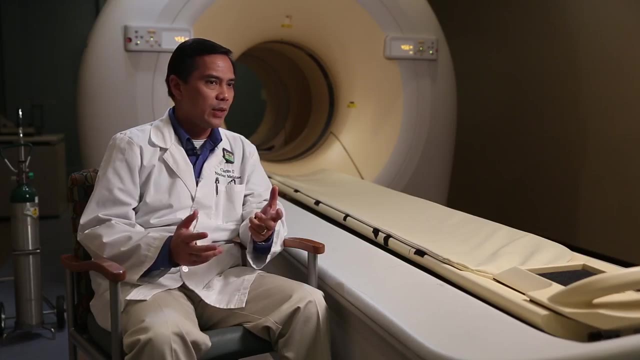 organs are not in the exact same spot in every patient, so you have to try to figure out. hmm, is that what I'm looking for, or is it not? What makes my profession different is that we get to play with a lot of technologies. 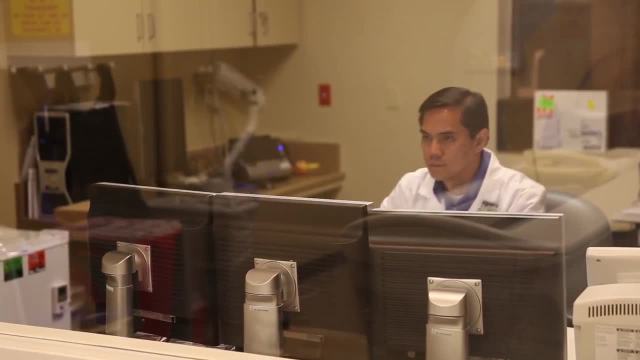 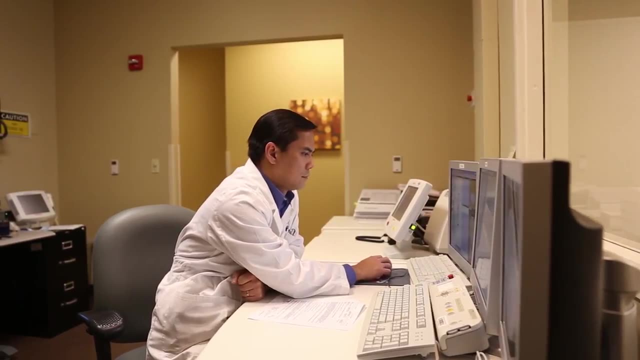 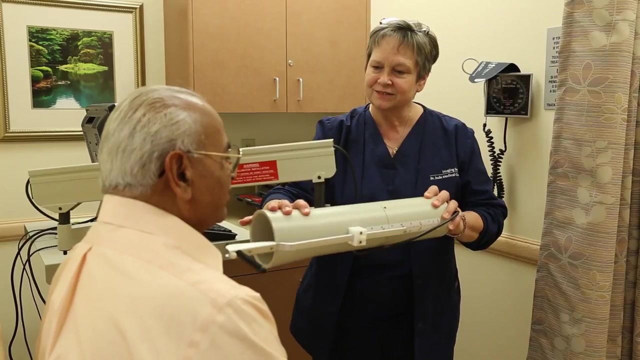 Right now we're in the forefront of fusion imaging, which is combining CT with nuclear medicine, MRI with nuclear medicine. Well, I've always enjoyed what I do and I think it probably is more because of the closeness that you can have with your patients. You have a real rapport with the doctors. that